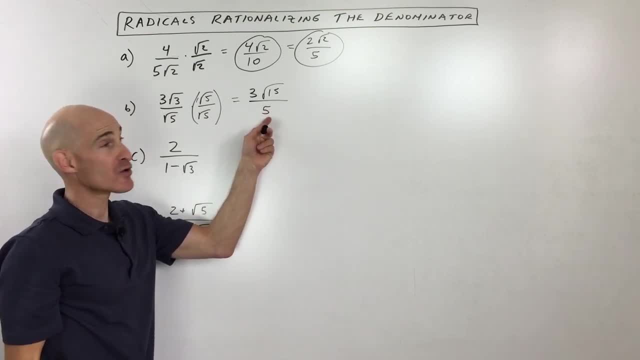 but we know the square root of 25 is just five. Notice, we got rid of the square root in the denominator. We can't reduce any further, so that's it. So you've simplified and you've rationalized that fraction. Okay, let's go to square root of five. 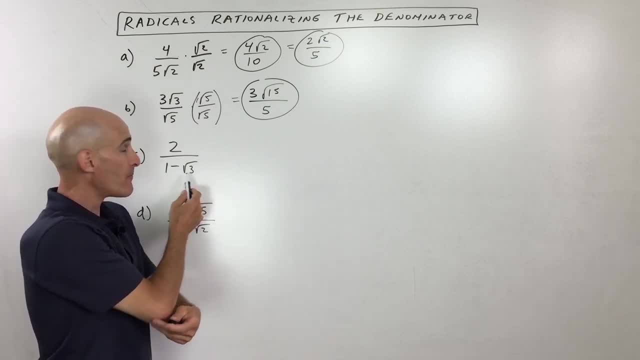 Some other examples. now, These two examples you can see. there's a binomial meaning. bi means two. There's two terms in the denominator. You don't want the square root in the denominator, but what we're going to do is a little different technique here. We're going to multiply by what's called the. 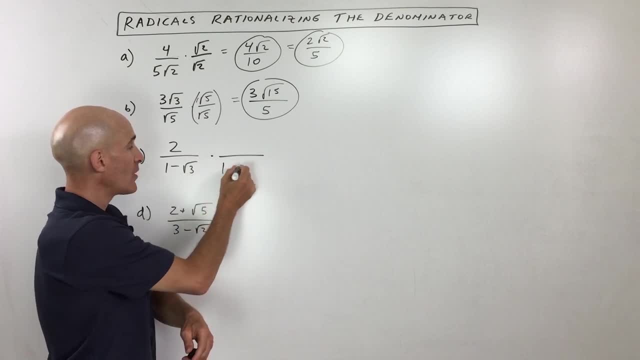 conjugate. So instead of multiplying by one minus square root of three, we're going to change that sign in between to the opposite, So one plus square root of three. If this was plus I would make this minus. Just change the sign in between the two terms. Again you can see we're multiplying. 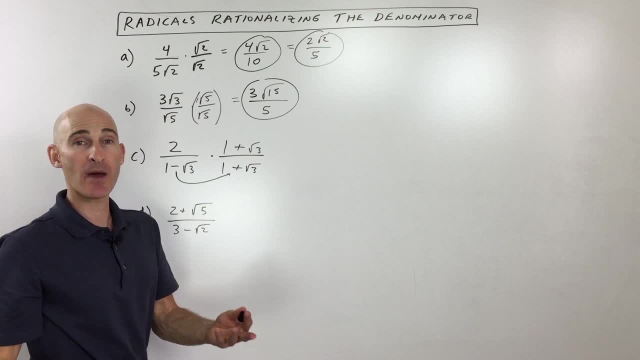 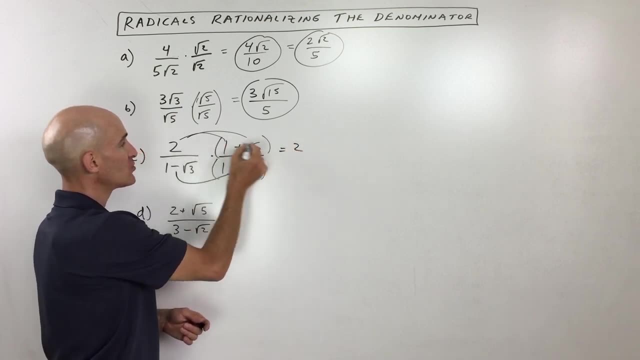 top and bottom by the same thing. so it doesn't change the value of the square root of five. It's just like multiplying by one. But what we're going to do here is we're going to distribute the two. Okay, so two times one is two. Two times the square root of three gives us two. square root of three. 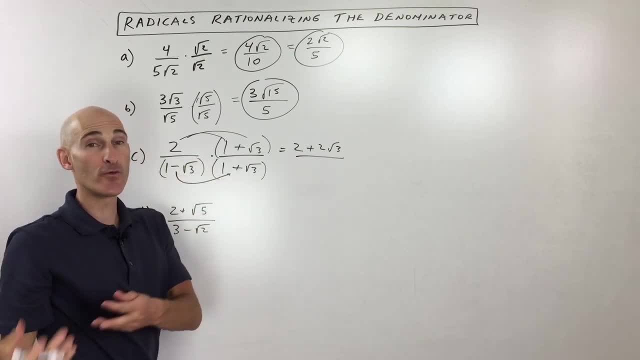 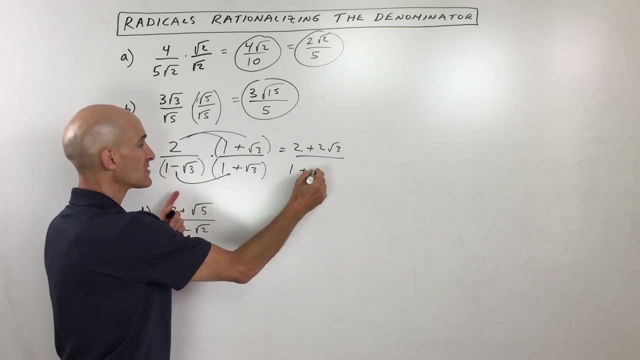 And the denominator. what we have is a binomial times a binomial We're going to foil, or you can do the distributive property twice. So let's distribute One times one is one. One times square root of three is square root of three. Negative square root of three times one is negative square. 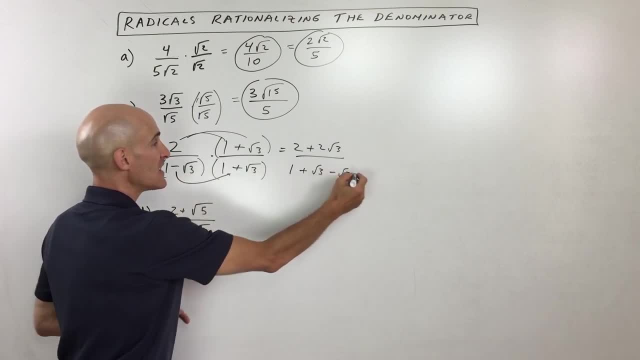 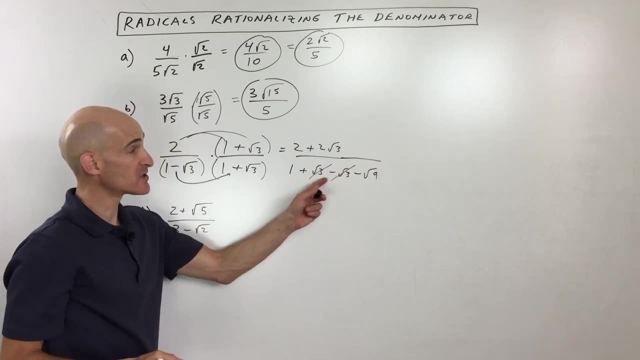 root of three And negative square root of three times positive. square root of three Is negative square root of nine. Okay, so notice what happens: Square root of three and negative square root of three, those cancel because one's positive, one's negative, Square root of nine is: 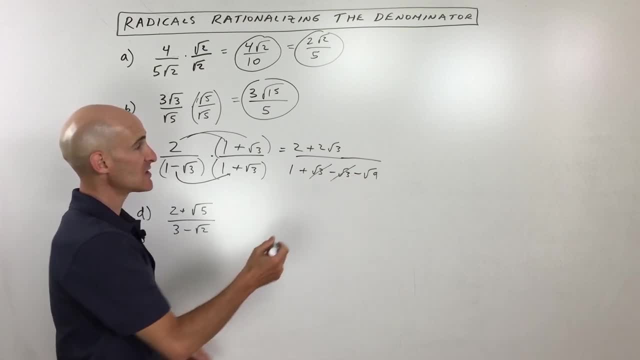 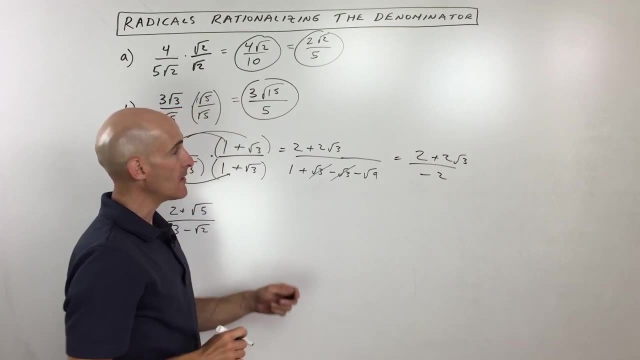 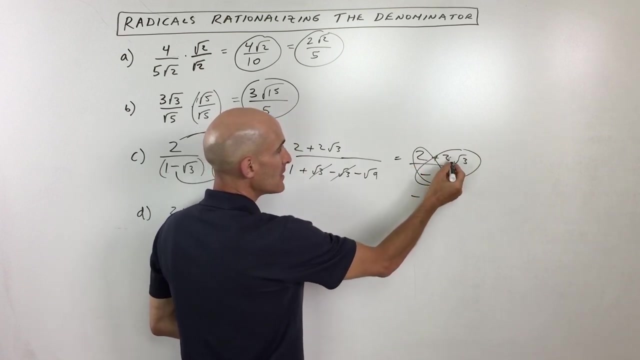 three times a negative is negative three. So one minus three is negative two And we're left with in the numerator two plus two, square root of three. Now what you can do is you can split this up, if you want, into two fractions. Two divided by negative two is negative one Over here. 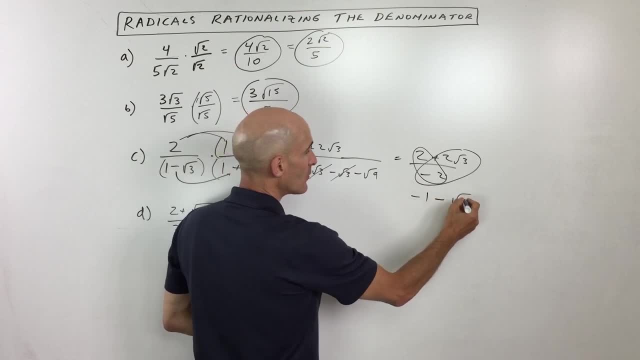 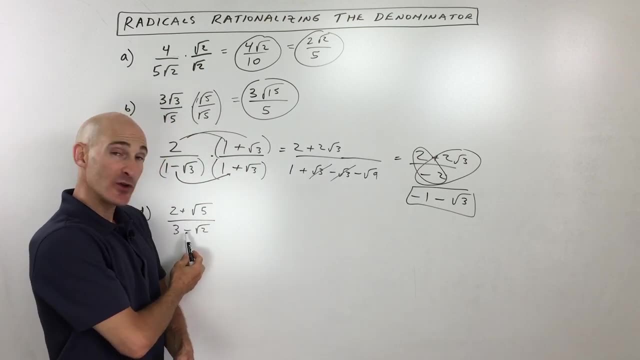 two root three divided by negative two, You can reduce. That's going to give you negative one or negative one root three. So we simplified that down a little bit further. Let's look at another example. So for this one again, we don't want that square root in. 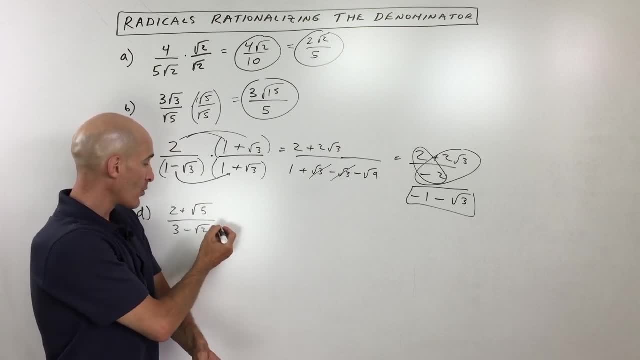 the denominator right. That's considered improper, but we have a binomial. So what we're going to do is we're going to multiply by the conjugate. So instead of being three minus square root of two, I'm going to multiply by three plus square root of two, And you want to do that to the numerator.